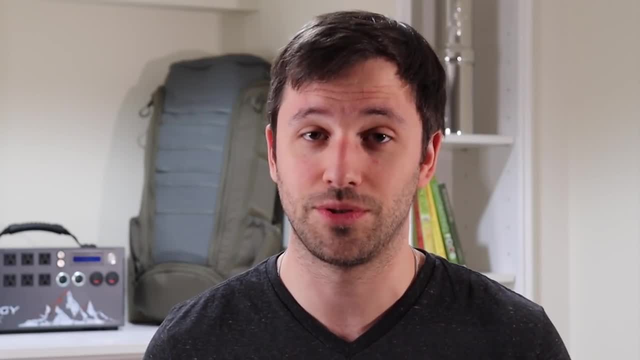 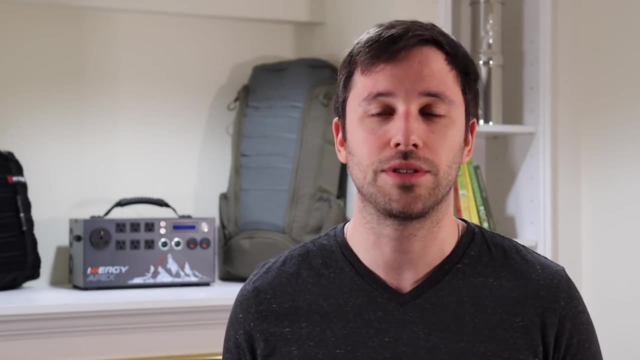 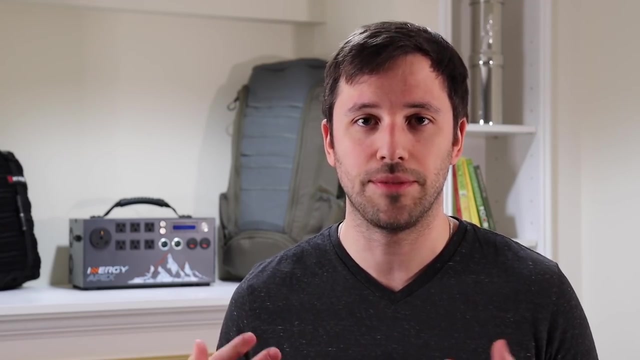 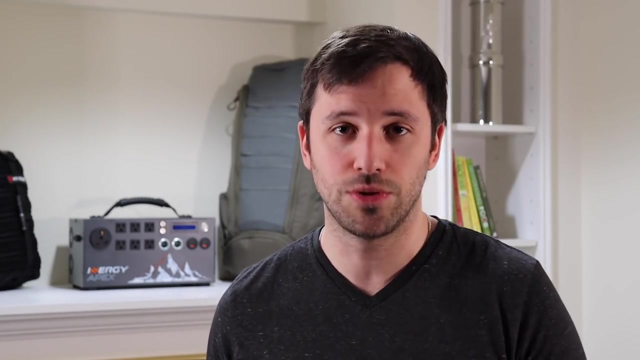 They're going to know how to do an overhand knot- unless you're still one of the cool kids using Velcro- But there's bound to be a time and place where those two knots are not going to cut it for you. They are not going to be able to handle the tasks that you might find yourself needing them to handle. Now, this is going to be one of the many videos that I include in my series. you know survival skills in 2022 that we should all master, So let's look at the three knots that I find the most useful and critical in a survival situation and what some of the applications would be for them. 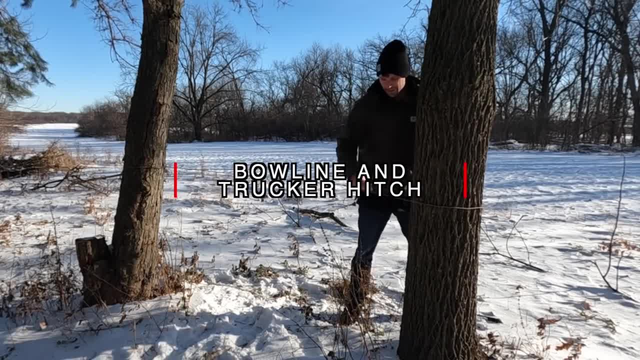 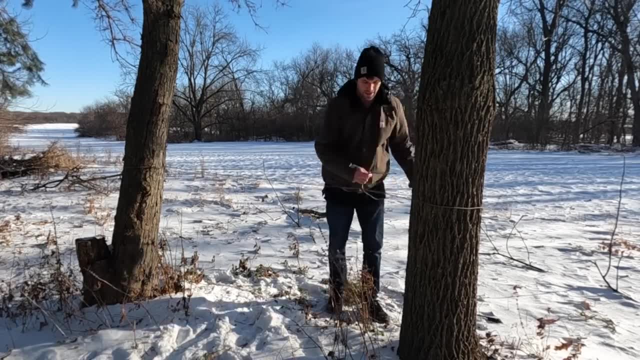 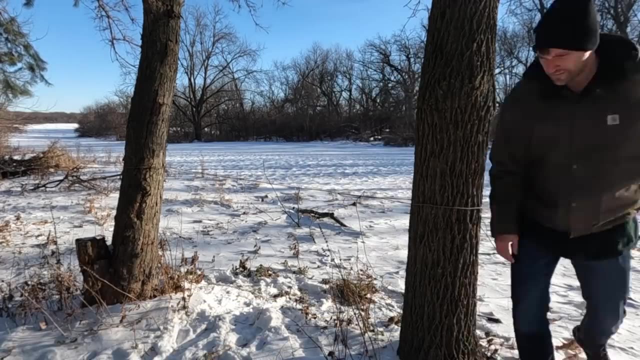 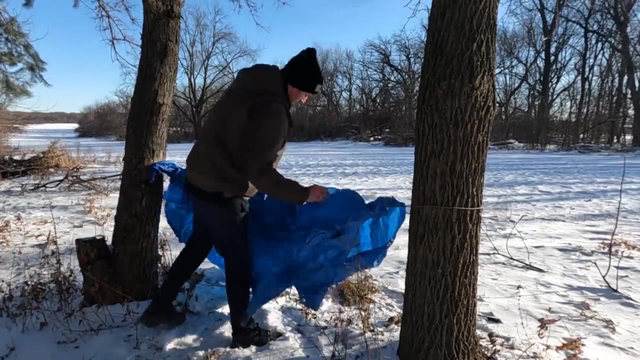 So the first two knots we have are the bowline and the trucker hitch. These two knots are a match made in heaven. If you need to build any kind of a shelter requiring a ridge line or a line that will go from one anchor to another anchor- in this case, two trees- this will prove as a foundation for you to build multiple types of shelters. This also works great as a clothesline where you can hang clothes and other types of gear if you need to keep something off the ground. The great thing about these knots as well is that they're able to be reused. This is not like an overhand knot. 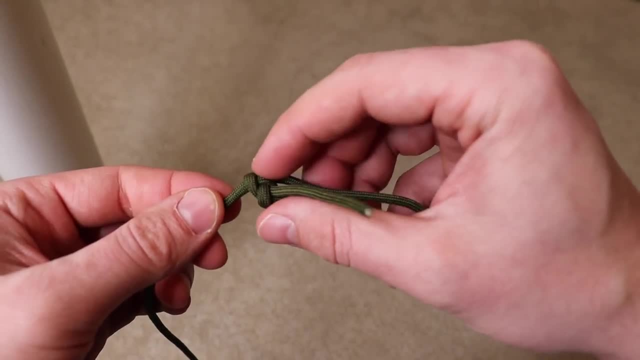 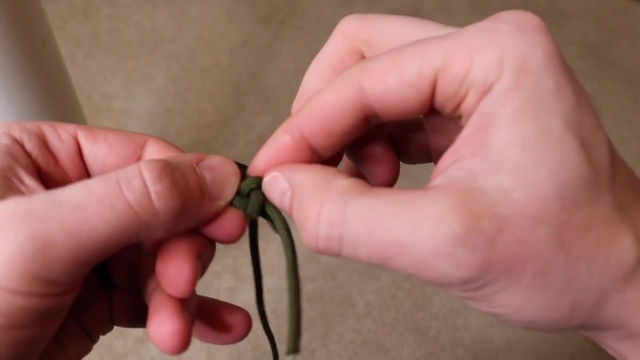 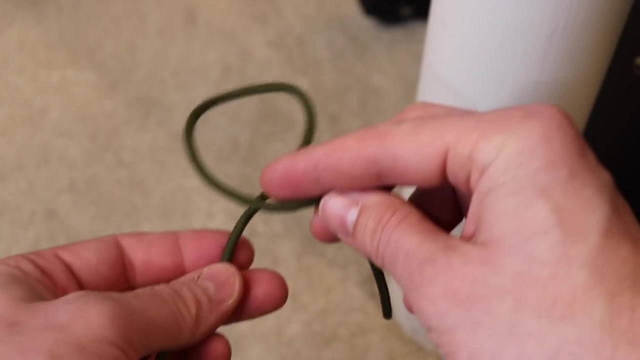 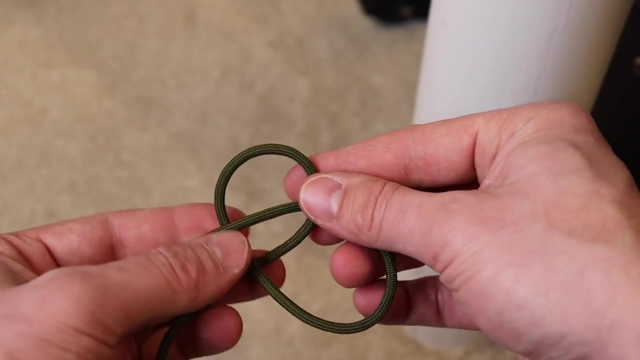 where the chances of you being able to release this easily are slim to none, especially in colder weather. If you see, here on the bowline, you're able to pull on this section here. Once you do that, it will release the tension in the knot and you'll be able to use this paracord for something else- To create a bowline. you will fold the cordage on itself. You will then take the free end and put that through the loop. It will then go under and over into the loop that you 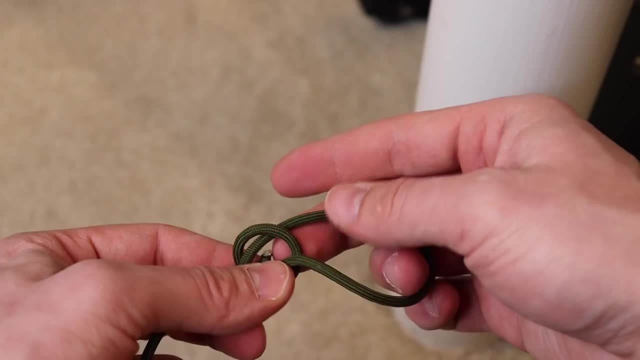 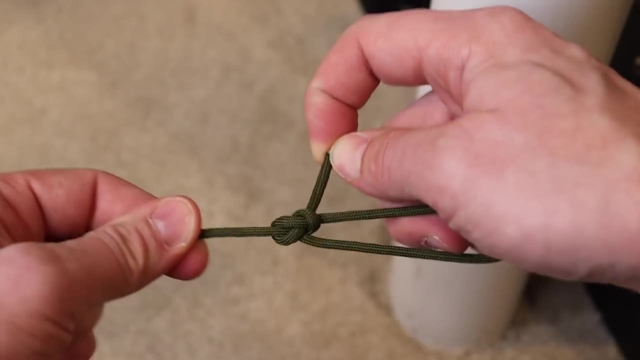 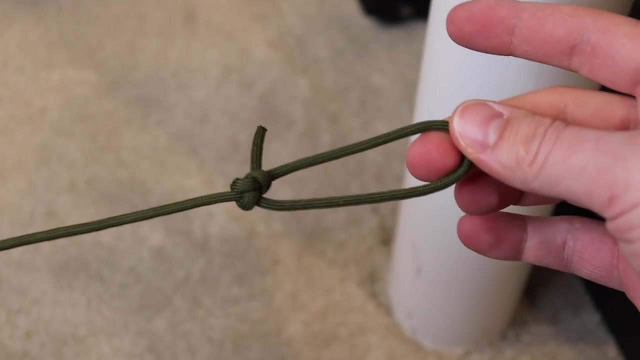 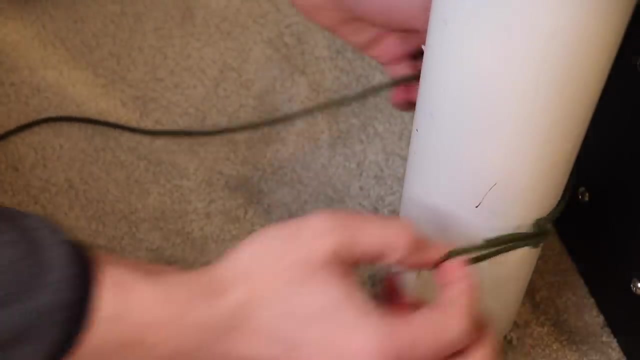 created at the beginning. This will then be your final chance to determine the size of the loop, so don't let it get too small on you. Pull it tight and you now have a non-slipping loop. In this example, we're going to use it as an anchor. So take your bowline knot that you just created. You're going to pull that cordage through the loop that you made against the first anchor. In this case, it's going to be the first anchor. 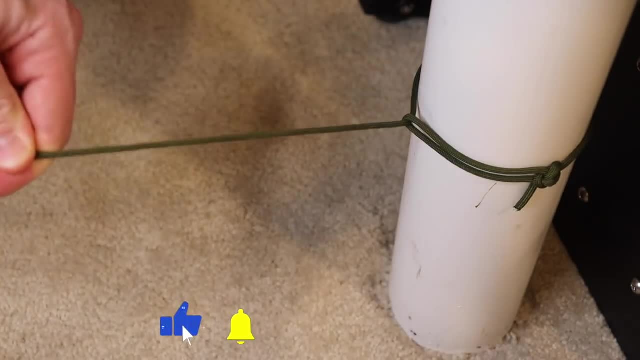 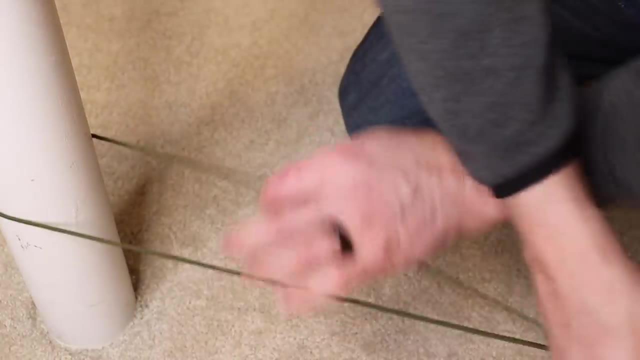 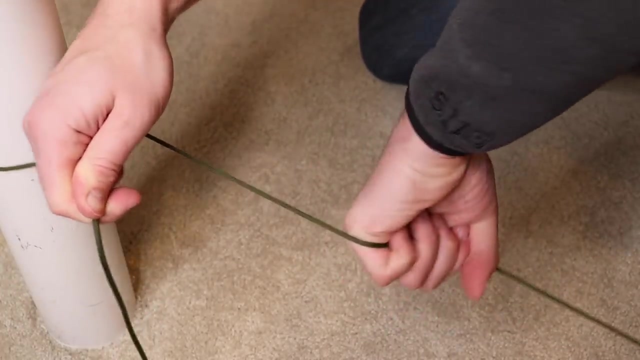 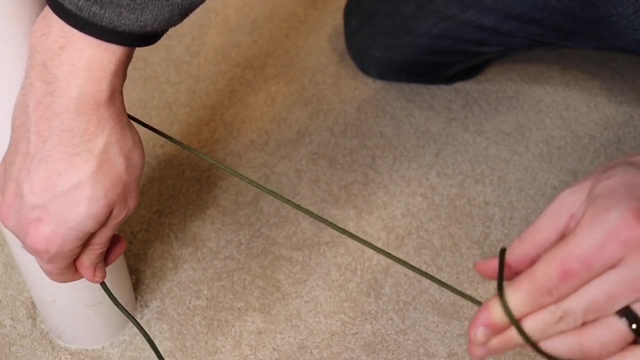 In this case, a pull. Now we're going to hop over to the other anchor where we'll apply a trucker's hitch. Now, at the other anchor point, we're simply going to pull the cordage around the anchor, and this is where we start to build the trucker's hitch. You're going to take your free hand, flip it upside down, grab the cordage, flip your arm back into a comfortable position upright. You'll now have a loop that you'll be able to get your thumb into and grab the cordage, pulling it forward to create another loop. 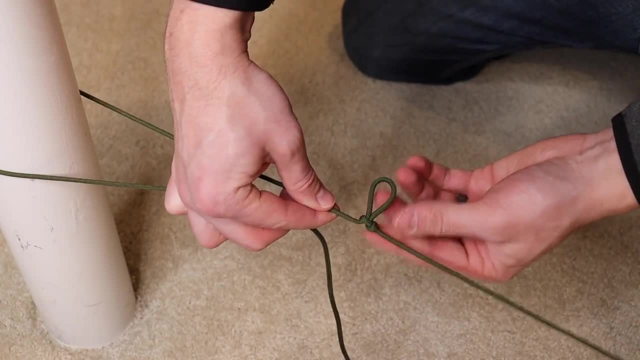 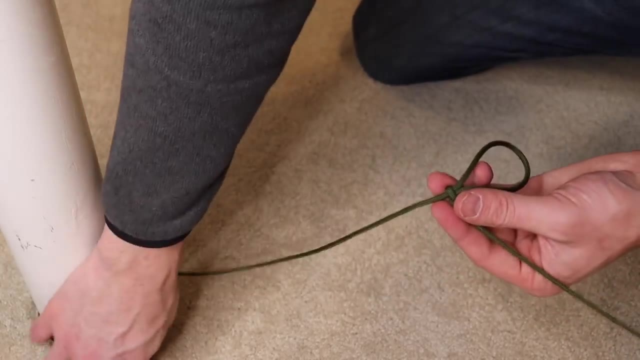 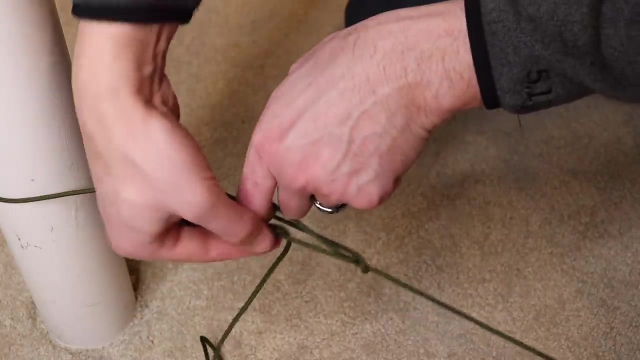 You can adjust this loop now, as you need to be able to get the other cordage through, because you're going to need to pull it taut and create the tension that you need. So once you pull that cordage through, you're going to pull on the loose end as tight as you need to, because we're about to lock that tension in. 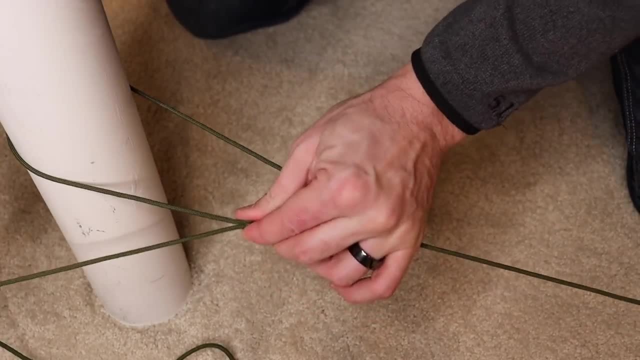 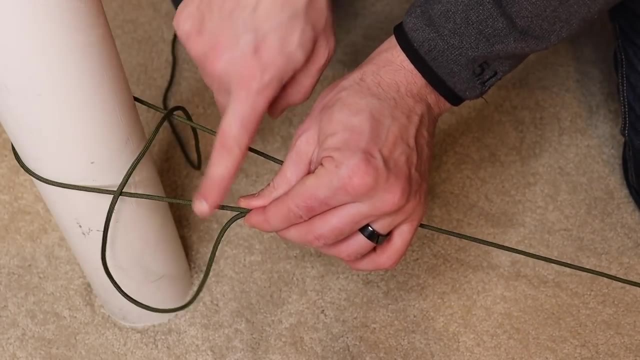 Take your free hand and pinch as shown. You're going to want to hold it in place. You're going to want to hold a lot of tension with your fingers here so it doesn't become loose. You'll now take the loose end of your cordage and pull it over your anchor point here. 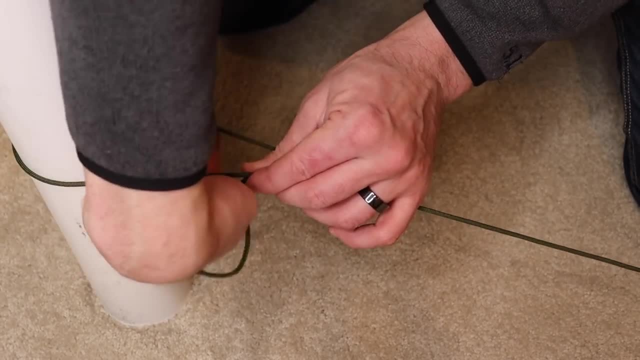 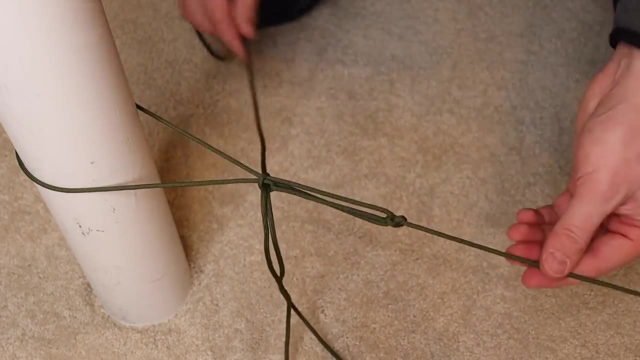 Keep a loop where you're pinching your fingers because you're going to get your free hand and snag that loose end of the line and pull it tight. This is going to be the knot that locks in the trucker's hitch and keeps the tension. 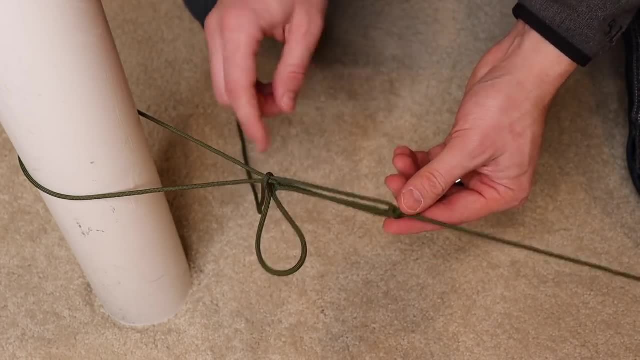 You could leave it as you see now, but if there was a chance your cordage could get pulled and loosen this knot, which is a quick release, then your entire ridgeline could come apart on you. So you'll want to hold it tight. 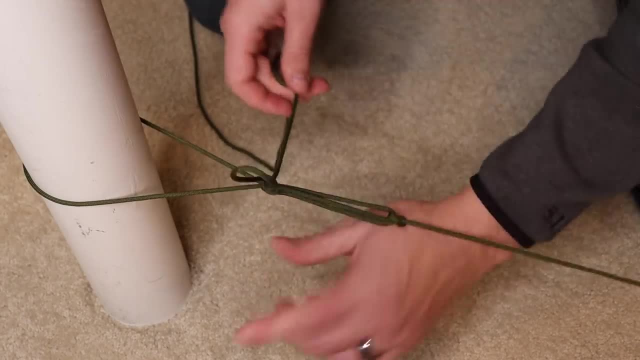 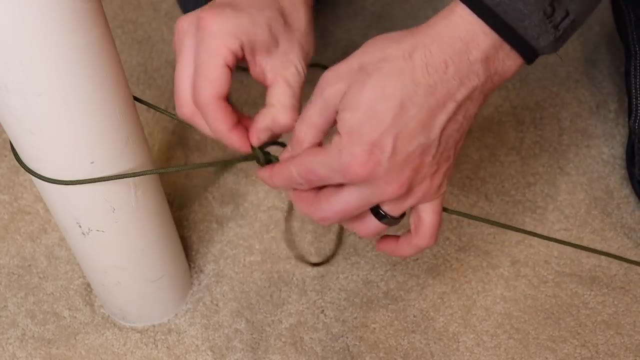 You're going to want to apply a safety and you can size this loop as needed. Some folks find it useful to hang things on this loop To take down the entire setup. just take your safety off and pull on the quick release. The entire thing will come down. 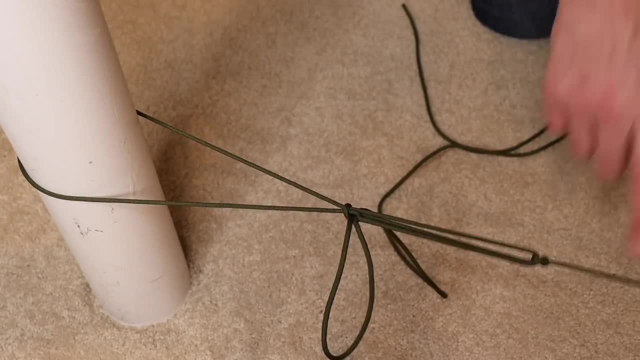 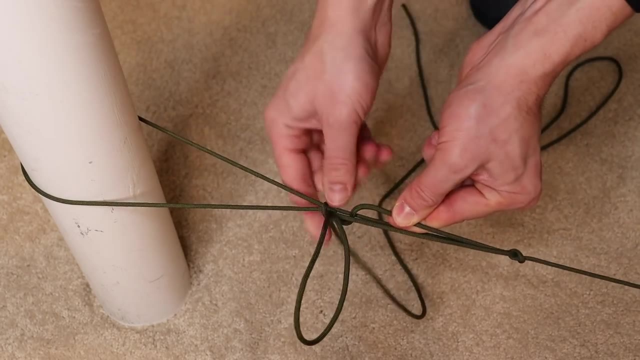 Now, in the event that your trucker's hitch has become loose, there is a way to tighten it up without taking the whole thing apart. If you grab the knot with one hand and you grab this section of cord here with the other, you will be able to tighten that by pulling it towards your second anchor point. 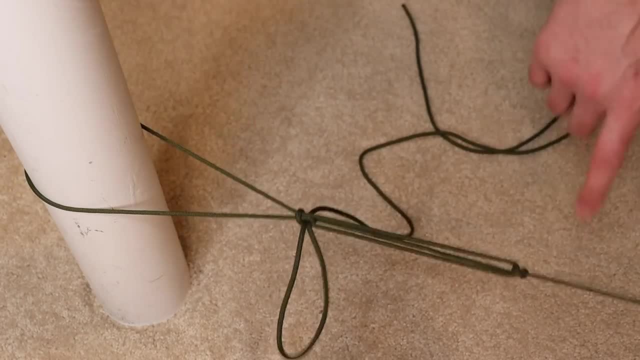 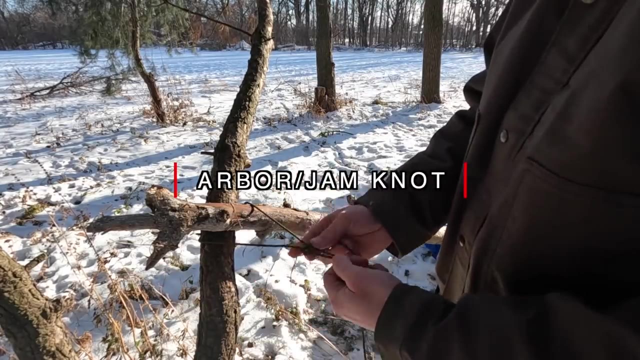 Just make sure to pull both so you don't unravel the trucker's hitch. The arbor knot, or jam knot, also known as the bushcraft zip tie, is extremely useful when it comes to building shelters or when you find yourself in need of joining two things together. 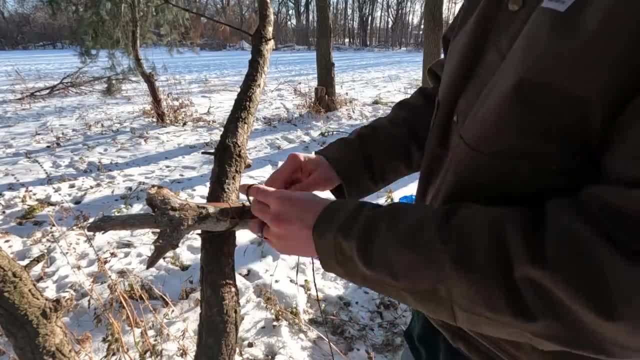 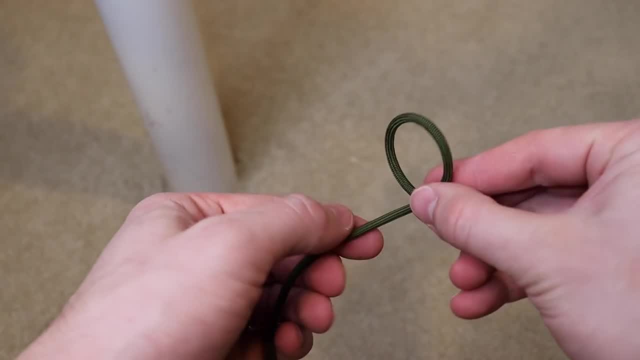 You can see in this example that I'm joining a large stick to a tree limb. To create this knot, you'll need to create a slip knot. Fold the cordage on itself to create a loop. Fold that loop on the cordage. 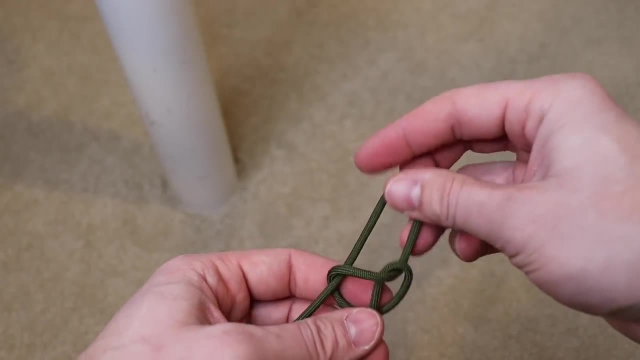 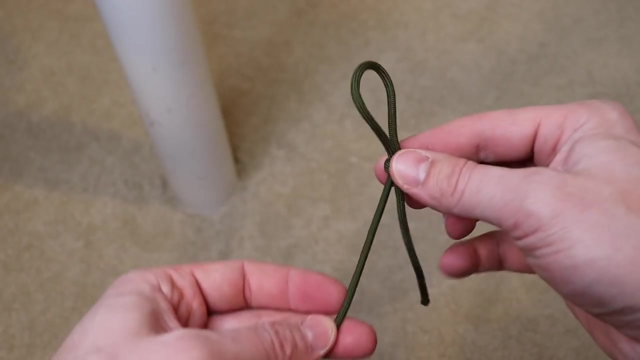 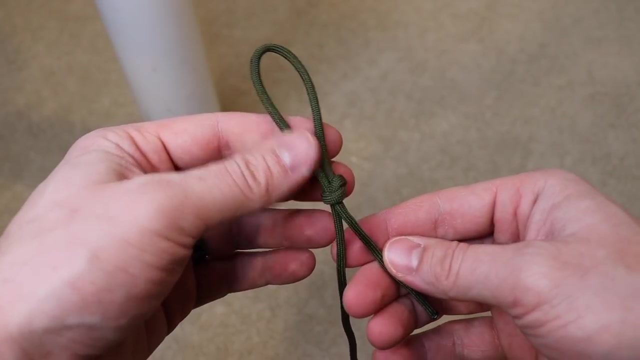 Then pull the cordage up, creating your slip knot. We're not done yet. We're going to need to create an overhand knot on the loose end that you see here. Just a single overhand knot will do. This will be a stop, so your slip knot does not come unraveled. 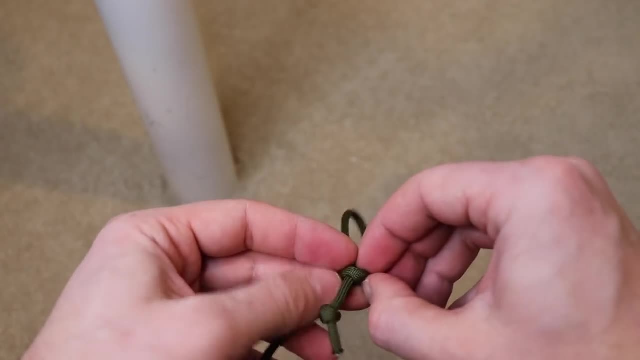 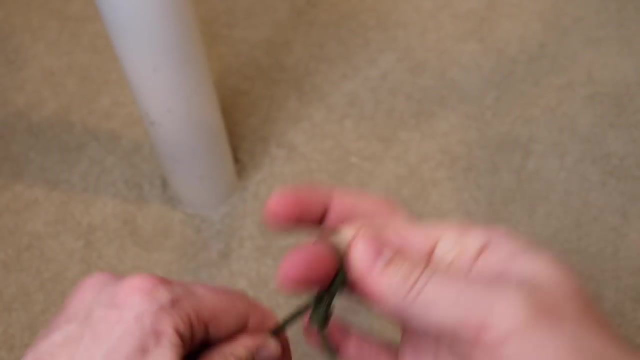 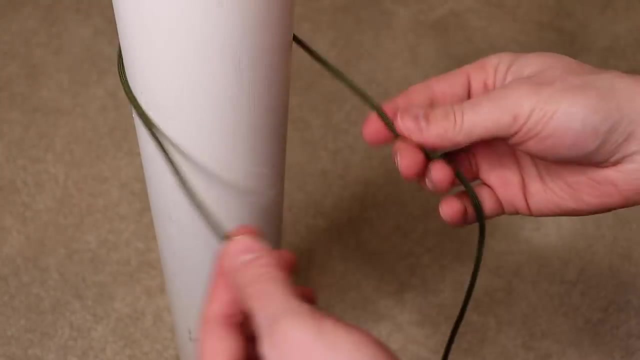 This method of creating this knot is great. if you have an object that you can slip this knot over and open it, the pressure to tighten it down, As you see it, can get pretty tight here. Now, if you need to apply this knot across an existing structure that you can't simply 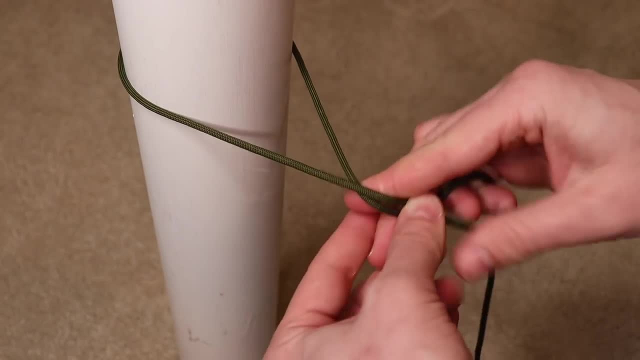 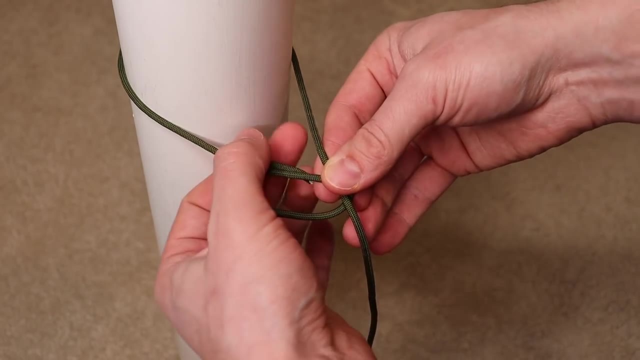 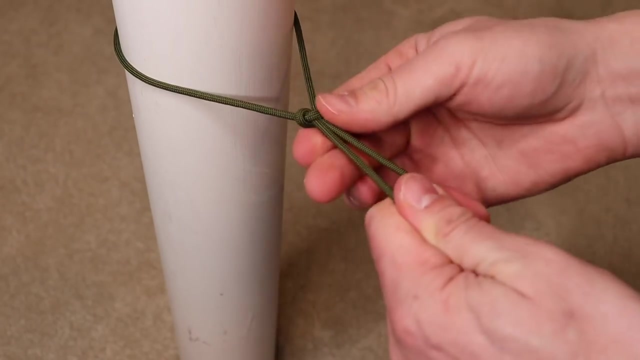 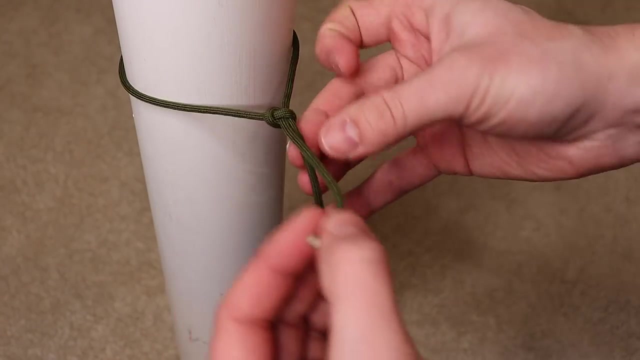 slip over. this is how you would do it: Wrap it around the object, bring your loose end over and to create your slip knot, you're going to do an over and through the loop Test to make sure that it slips. create your overhand knot as. 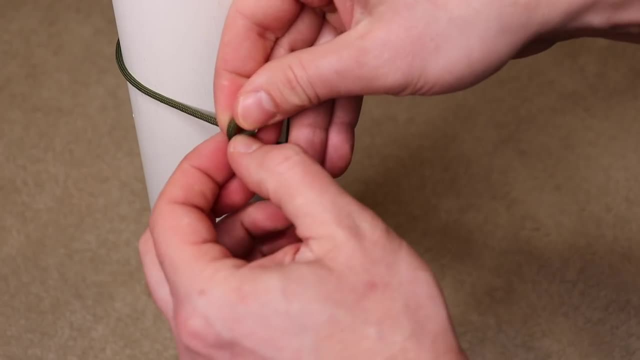 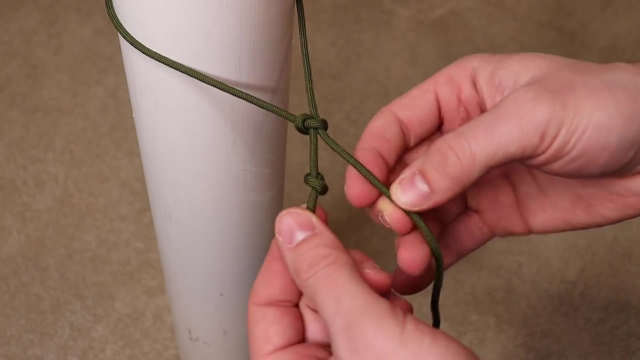 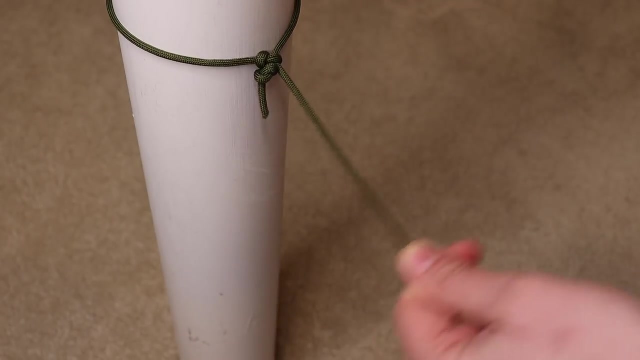 the previous example showed, and tighten down on the object or objects as tight as you need. It's showing a little bit of slippage here, but that's because this is a pole. This won't slip nearly as much if you do this on a stick, for example, Once you. 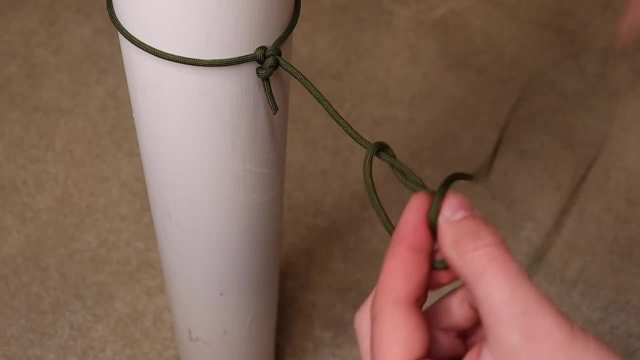 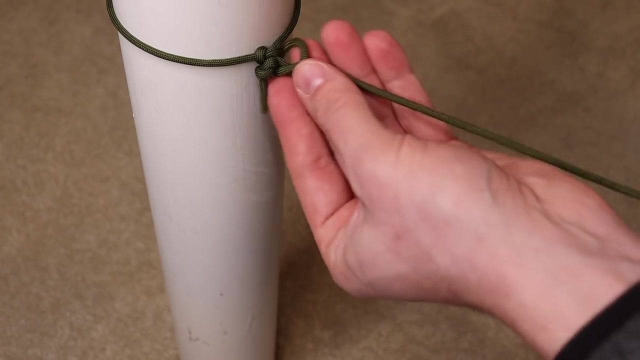 have it as tight as you need. create another simple overhand knot, and you're going to move this into position as far up as you possibly can so that this zip tie will not come undone. You could cut the extra cordage off here and use it on. 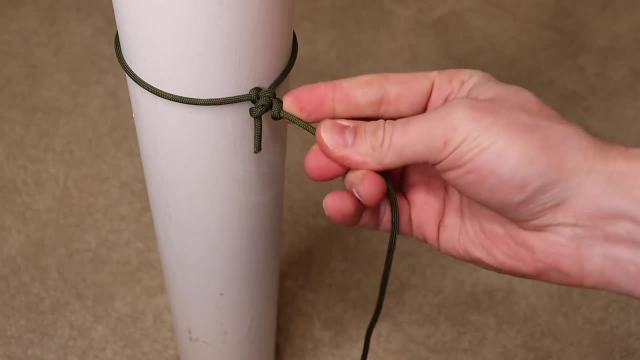 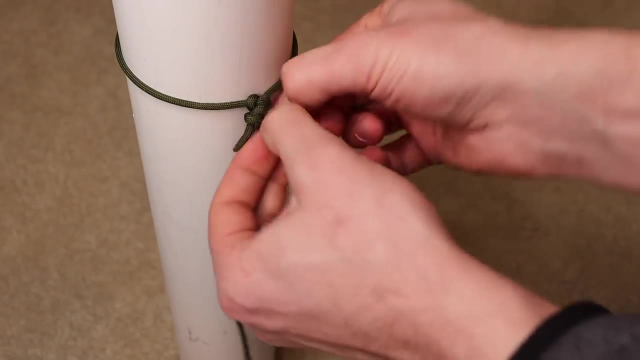 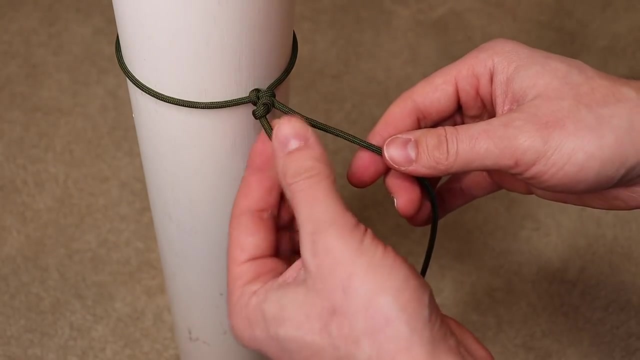 something else. If, for any reason, you need to take this off or want to reuse the cordage, just undo the last overhand knot and pull on the initial overhand knot, which is called the key. By pulling on this key, it will essentially release the tension on the knot. 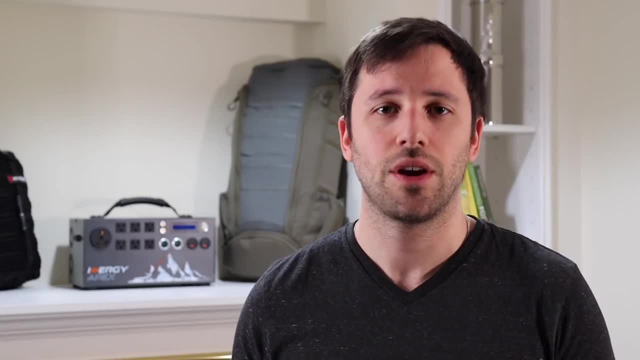 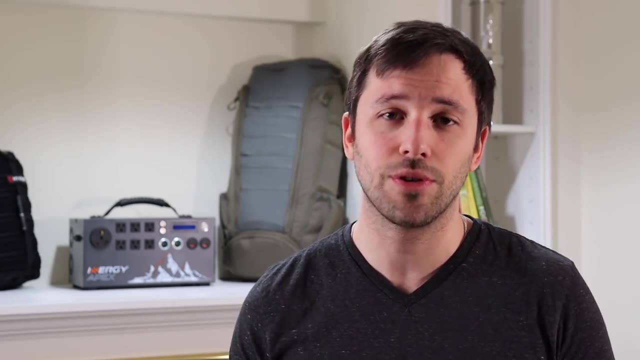 Alright, folks, let me know in the comments what's your favorite knot. What do you use it for? What do you think should have made the list, or maybe not made the list? Also, if you're interested in this kind of content, don't forget to comment, like and subscribe. 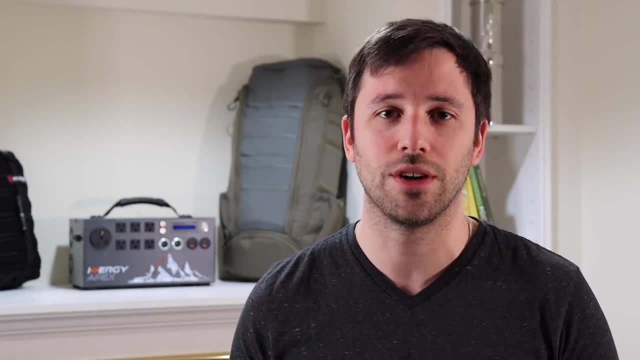 It helps the channel grow and you'll get more videos like this every time I upload a new video and you'll get notified when I come out with more videos. Until next time, folks. 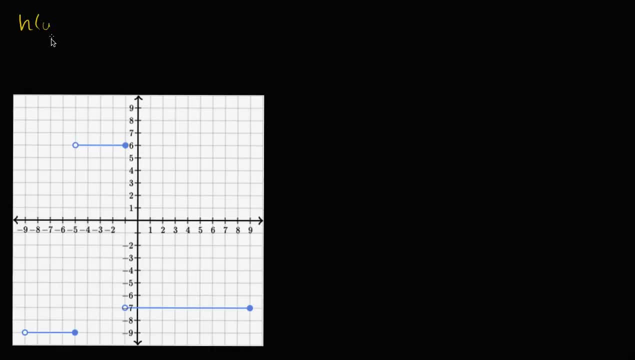 By now, we're used to seeing functions defined like: h of y is equal to y squared, or f of x is equal to the square root of x. What we're now going to explore is functions that are defined piece by piece over different intervals, and functions like this: 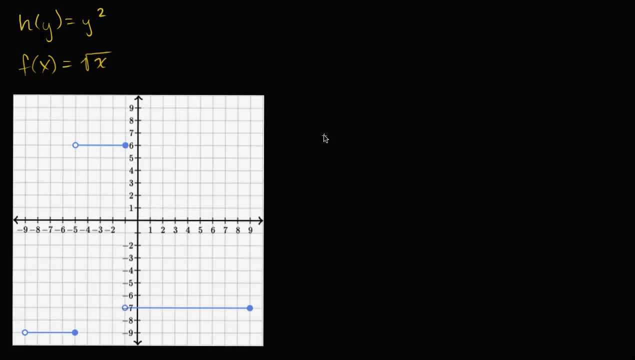 are. you'll sometimes view them as a piecewise or these types of function definitions. they might be called a piecewise function definition, And so let's take a look at this graph right over here, This graph. you can see that the function is constant over this interval for x, and then it jumps. 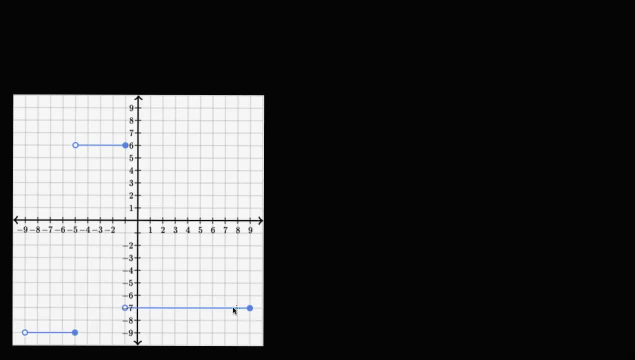 up to this interval for x and then it jumps back down for this interval for x. So let's think about how we would write this using our function notation. So if we say that this right over here is the x-axis, and if this is the y, 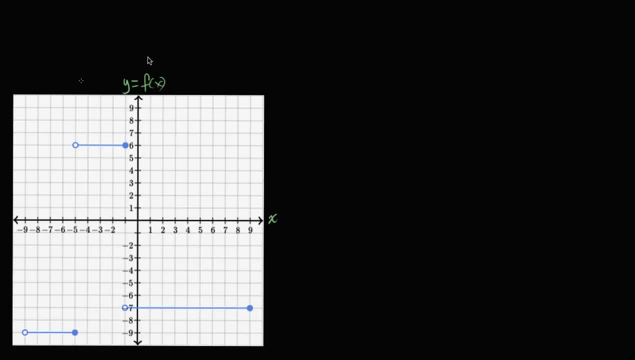 is equal to f of x axis, then let's see our function f of x is going to be equal to. let's see there's three different intervals. so let me give myself some space for the three different intervals Now. this first interval is from not including negative nine. I have this open circle here, not a closed in circle, so not. 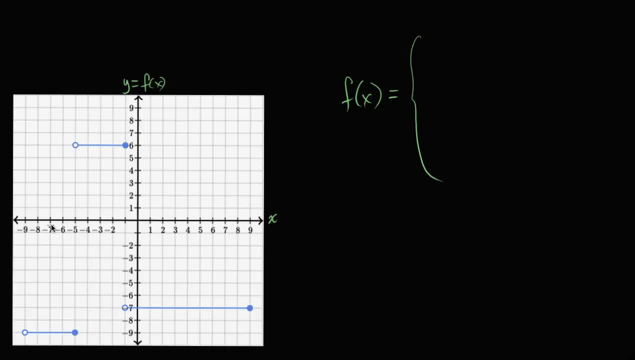 including negative nine, but x being greater than negative nine and all the way up to and including negative five. So I could write that as negative nine is less than x, less than or equal to negative five. That's this interval, and what is the value of the function over? 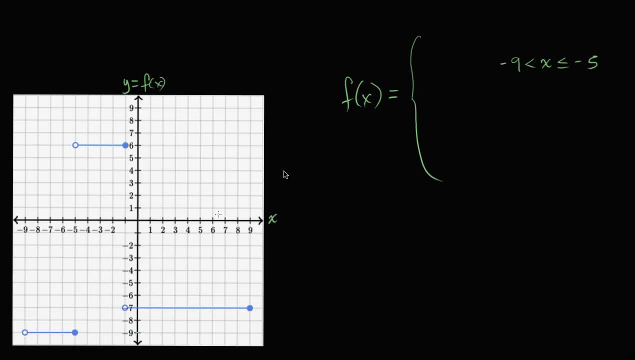 this interval. Well, we see, the value of the function is negative nine. It's a constant negative nine over that interval. It's a little confusing because the value of the function is actually also the value of the lower bound on this interval right over here.